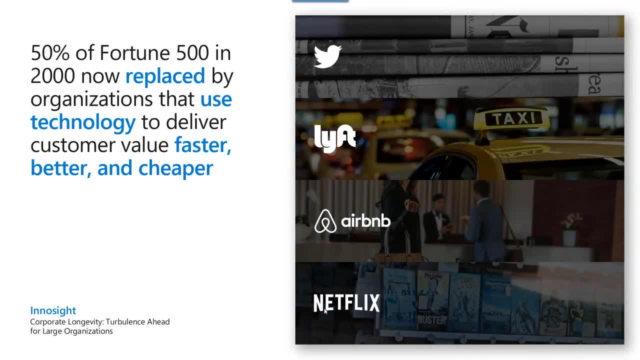 So for those they don't know about the Fortune 500, there is a magazine in the US where it lists the top 500 companies based on the fiscal year revenue. So 50% of these companies has gone. It does not exist. It has been replaced by companies that use the technology to deliver. 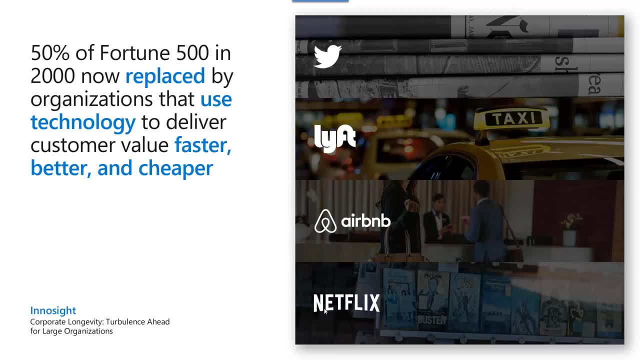 the customer value faster, better and cheaper. If anyone remember or knows the Black Poster company, which was one of the top companies that renting movies in the US In 2004,. it has about 10,000 stores, 5,000 of them only in the US. It has revenue in billions, This company. 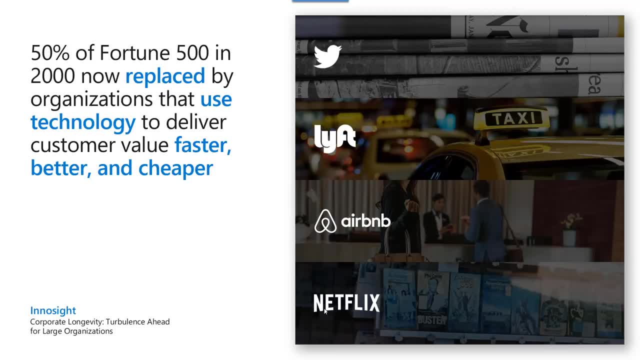 has been kicked out of the market and replaced by a startup company. This company called Netflix back in 2010. in the time, In 2010,. Black Poster has big problem and after a couple of years, it's completely gone. As we can see, it is not just that this company 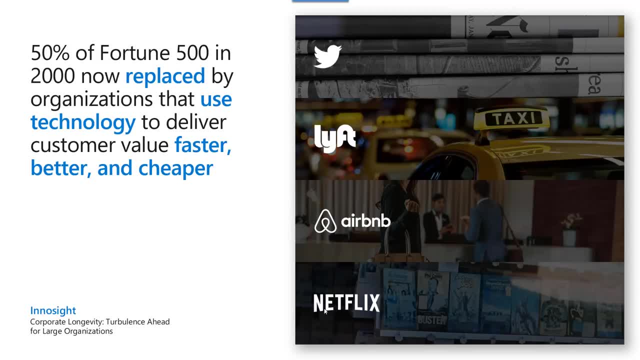 affecting some of the revenue for the competitor. It lead to that this company completely vanish. This is why technology changing the way that we doing our business. It changing the way that we deliver our services for our end user, how we deliver the products. What is the value for? 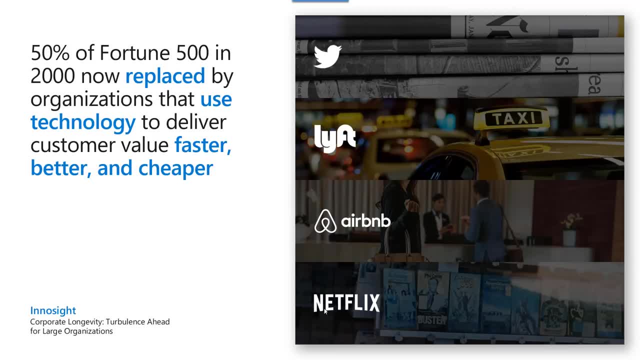 Black Poster for 10,000 stores in the US, while Netflix delivers the movies using an app on the TV for everyone in his home. And for those company that they don't understand the digital disruptions that happening, they will face the same fate. This is why we usually say that the 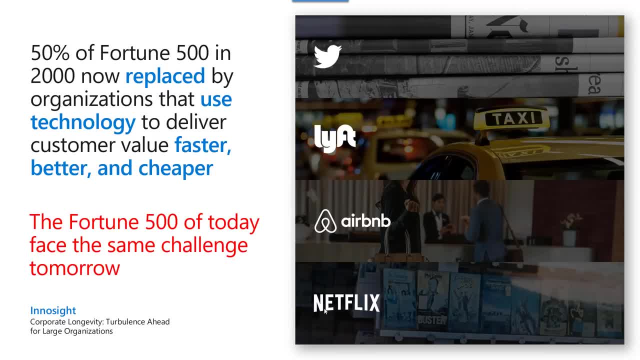 current 500 today. they are not going to be the same fate. They are going to be the same fate. We'll face the same challenge tomorrow if they don't understand the digital disruption and how to use the technology to get innovation. So this is why usually I will say business and technical. 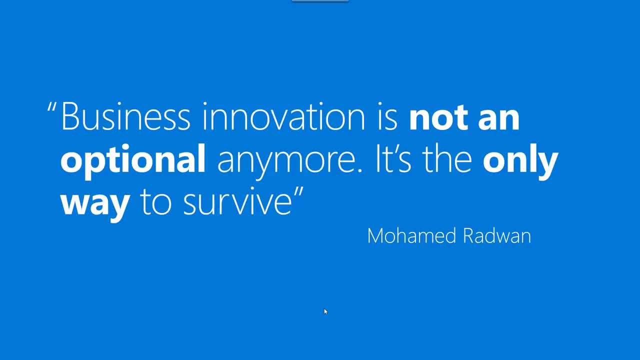 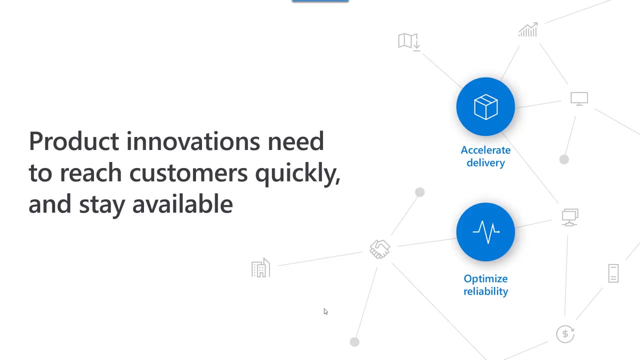 innovation. it is not an optional anymore. It is the only way to survive. As we saw, it is not just affecting that the companies may get less revenue. It just may lead to the company to be completely out of the market. Since we understand the importance of the innovation, we need to understand that innovation needs to be. 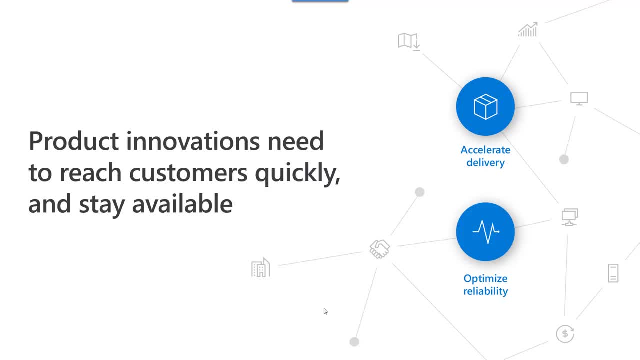 delivered quickly to the end user, at the same time reliable. So it's very important to give the end user quickly the value And at the same time, the value or the services available is secure. It doesn't have many problems. So because at the end, 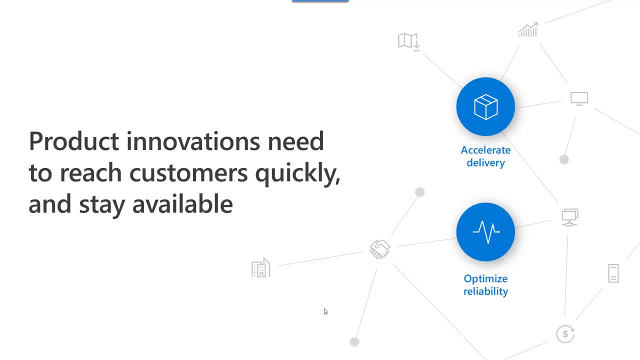 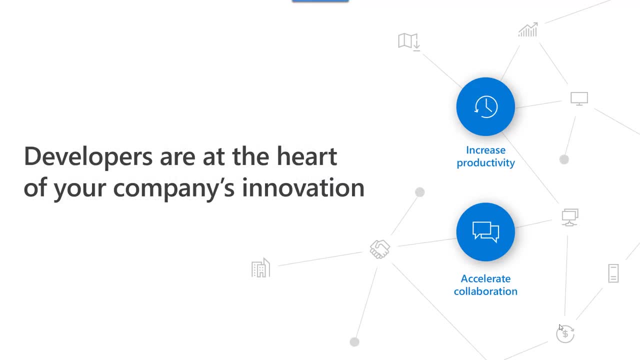 if I deliver quickly without reliability, then I lose the brand, I lose, the customers I lose, and all of that And because we are living in a technology driven world, so developers are the heart of the company, innovations It, and it's very important to provide the tool for the developers that increase their productivity and 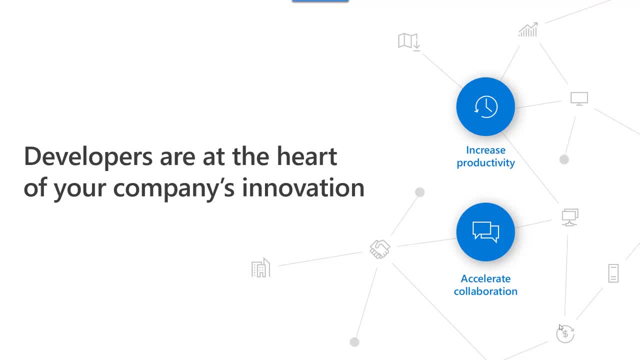 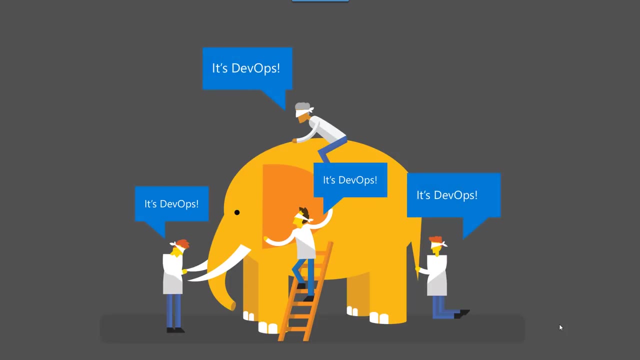 accelerate the collaboration between them So it can help for bringing more innovation to deliver the value quickly with high reliability. DevOps: If we ask what is DevOps, probably we will get different answer or different definition about DevOps. So for some people it's all about cooperation between development and operation. Some other is 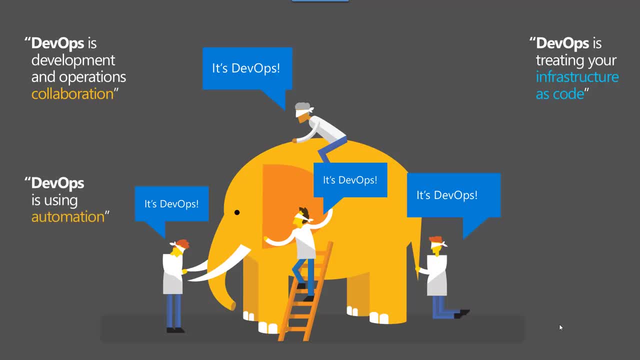 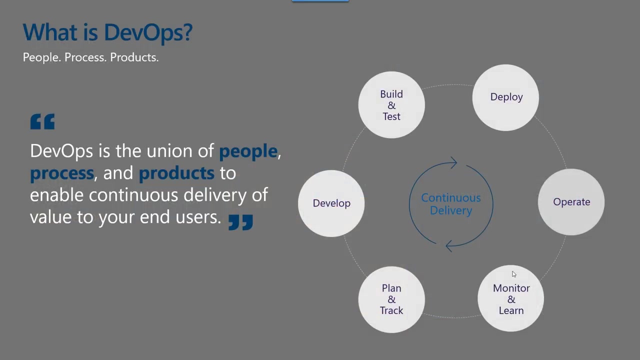 infrastructure as good, and for other it's all about automation, While others believe that it's a culture change. far helps to build and train the team. small deployment or frequently deployment can ban for operation or it's a job title. So what is DevOps? 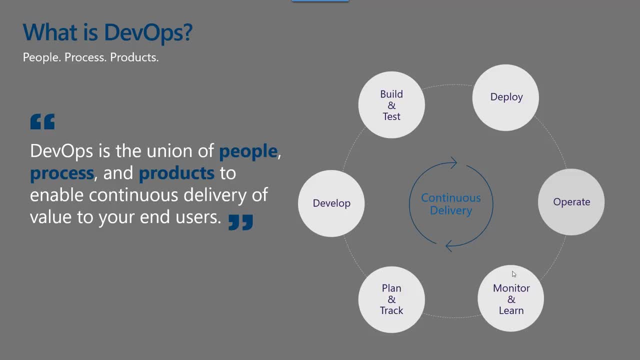 DevOps. none of the previous DevOps is not continuous integration or not continuous deployment. Of course all of that is part of the DevOps, But DevOps is more wide than this. So it is all about union or the integration between people, process and products to deliver continuous value to the 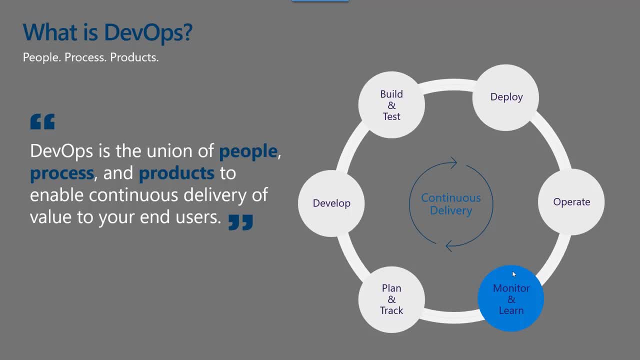 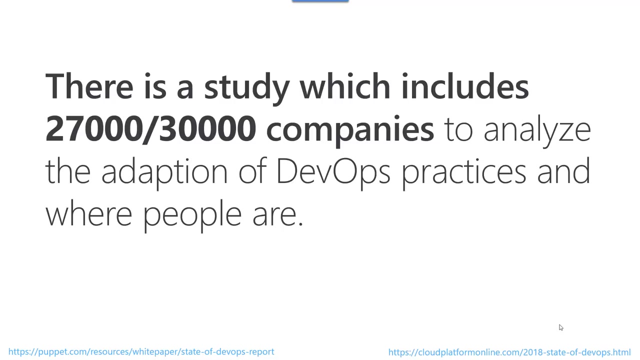 end user. so it it just look at the complete end-to-end for the software development and delivery and this is the main idea of the devops: deliver quickly with a high reliability for the end user. there is a study which includes around 27 000 to 30 000 companies to analyze the their. 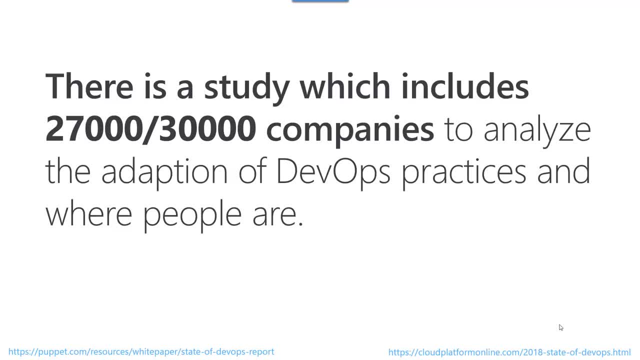 adoption of devops practices and where people are the study done by two organizations. one of them is dora, or devops research and assessment, which is non-profit organization and provide academic research, and the second one is puppet, which is a software company that provides a configuration management tool, and the numbers is is almost close to each other. so let's look at. 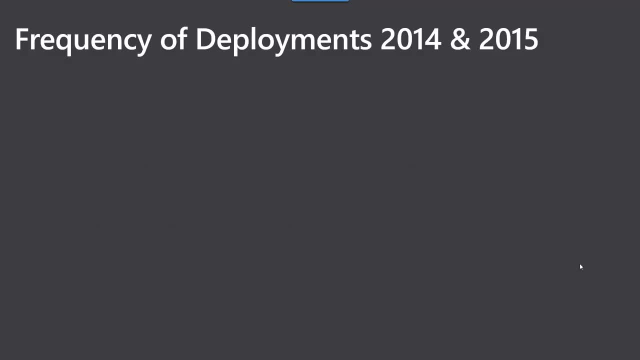 some of the results. the study has many useful information, but let's take one of the important metrics, which is frequency of deployment in production. so they found in 2014 the following value for frequency of deployment and production: in 2015, they found that the frequency of deployment 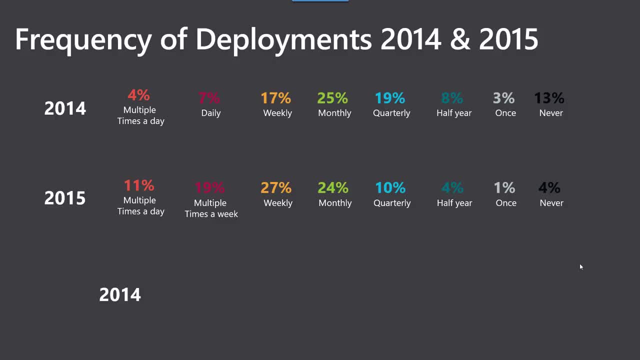 has been equal to a maximum increased with these values. so the increase was around 17 percent from 2014 to 2015, 40 percent in 2016 and around 60 percent in 2017. so, as we can see, more company are going to more frequency of 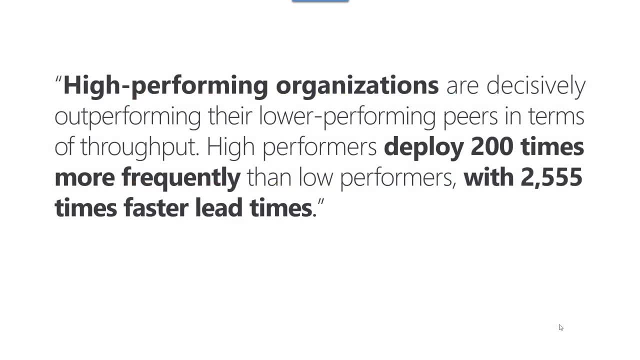 deployment in production. so if we look at the study and to see the company at the top, they found that it deployed 200 times more frequently than the company at the bottom. for example, if the company at the top is deployed in production every one day, then the company at the bottom will deploy. 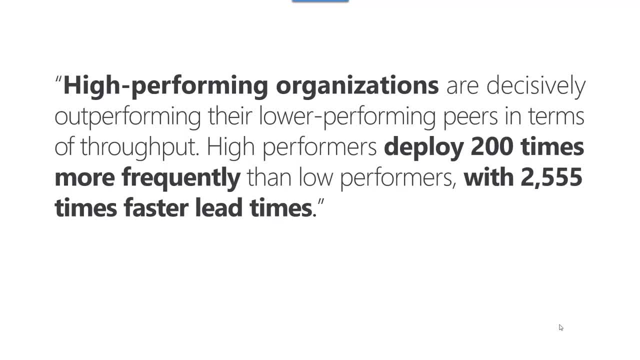 every 200 days in production. also, the company at the top. it has faster lead time, with 2555 more than the company at the bottom. the lead time is the time or the duration between working on the requirement from the beginning until deploying this requirement to production. so, for example, if it's required one hour, 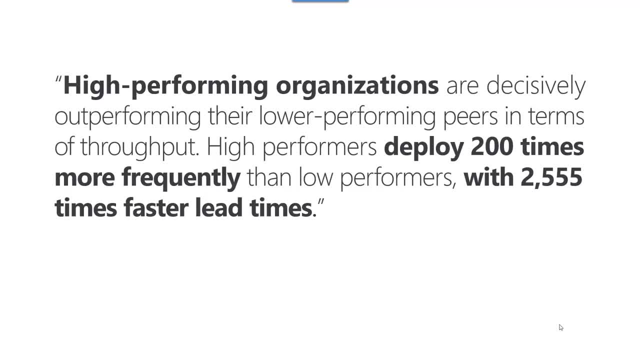 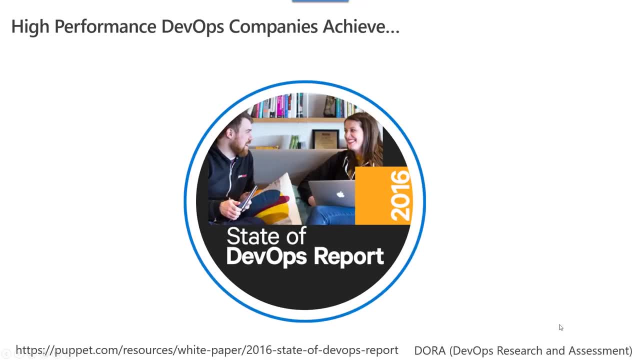 from the beginning to the end to complete one requirement. the company at the top will take one hour, then the company at the bottom will take two thousand five hundred hours. so what they found? they found that the companies that implement high performance first. they exceed two times their profit, market share and productivity goals. 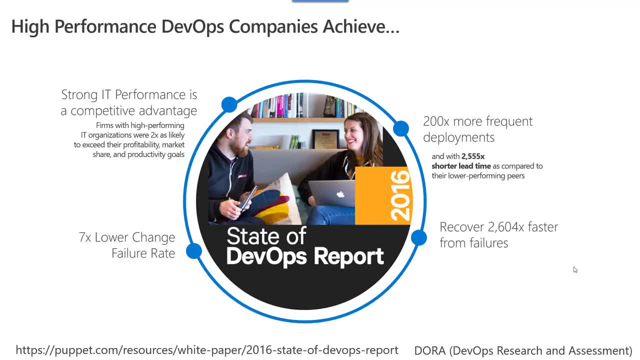 they don't fail and if they fail, they fail less seven times of the company at the bottom and they recover 2600 faster from failure. i can spend all the day talking about this point, the main idea of recovering from failure. let's say, for example, after: 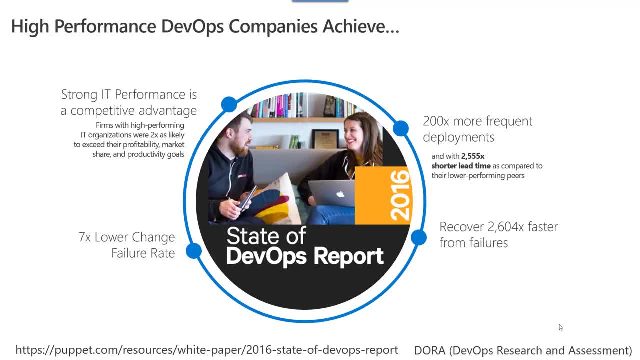 the maintenance of a few months of the application after 2 years of the production, or 10 minus than the market to start from low 8 to 8. they couleur by the Api 있어 the new based modelという. they deploy the new version in production. the application is not working properly, and you know, and they need to fix that, or 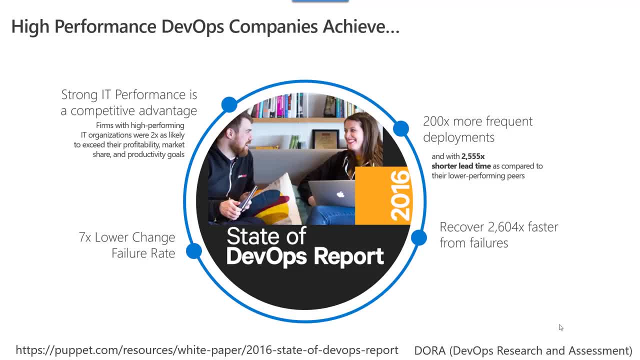 hours. and why this? the main idea that the company at the top, they are impressed, the failure they are not afraid of the failure fail fast. they fail many times and they learn from their failure. they understand how to master this failure. so, but for company at the bottom, they keep fighting to prevent. 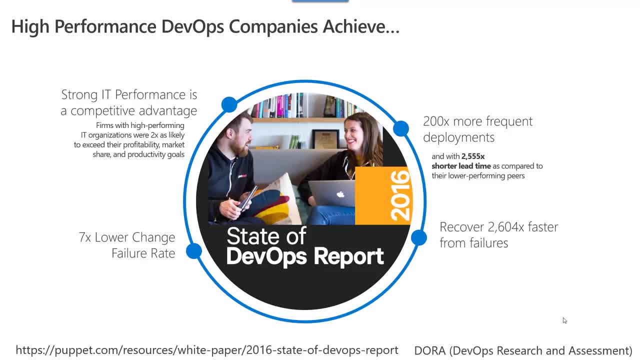 the failure. they put all the effort to prevent the failure from happen. they put many documentation like disaster recovery, you know many documents planning for dealing with the failure and when the failure happen they bring all the documents, try to fix that and they are struggling to fix a problem. and it takes time to fix a problem because they are not ready. but for the other, 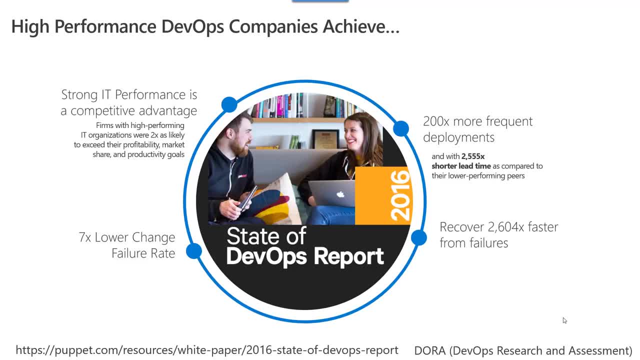 company. again, they don't prevent the failure. they keep measuring the failure rate and the main time to, to detect, the main time to recover, and this measure which shows them if they are on the right track or not. and after the preventing the failure, they have less failure rate. this is 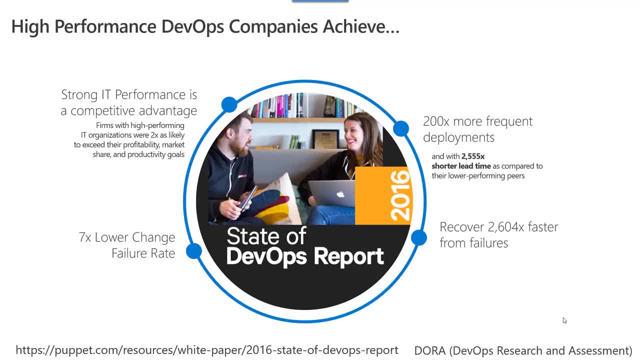 why some companies, uh, created some affiliate frameworks to, like netflix, created chaos, monkey where it's, and it's an open source on github where they can make failure for the system because their system it doesn't fail, you know. so they need to make that in purpose so they can train. 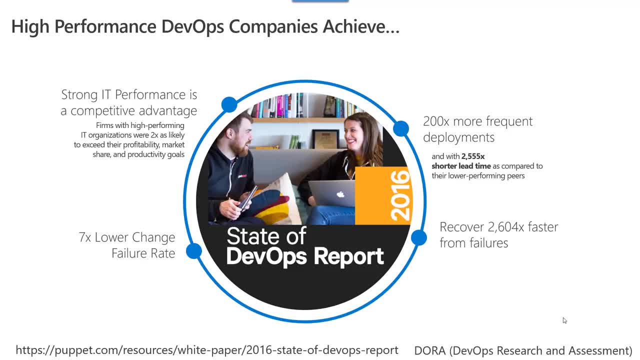 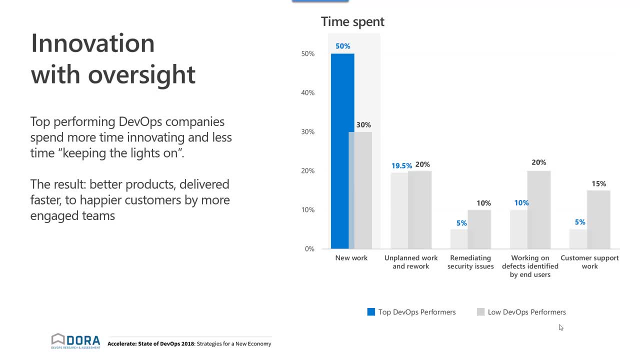 on how to interact or deal with with the failure. so if we look at the innovation with oversight, so top performance devops companies spend more time in innovation and less time keeping the lights on, as we have more time because we don't fail and if we fail we recover very fast. so 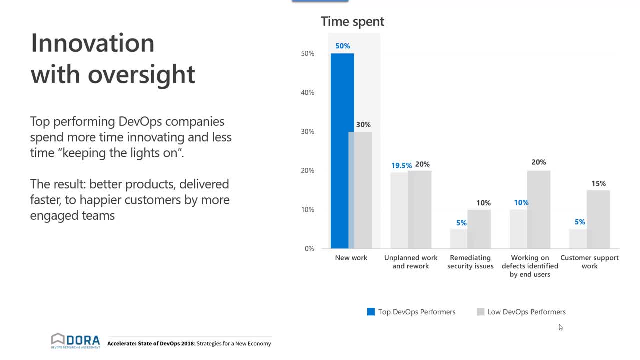 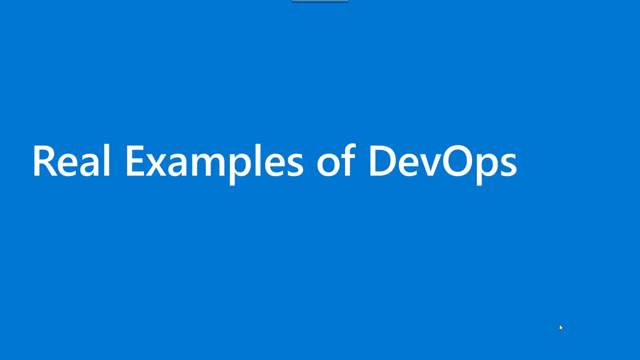 they this time that we, that other company, used to recover from failure and just covering all this problem. the top companies. they just use this time in innovation, in new work and this bring more value to the end user and give the end user the value very quickly. real example of devops. so is there any real story? so we can see, yes, if we look at. 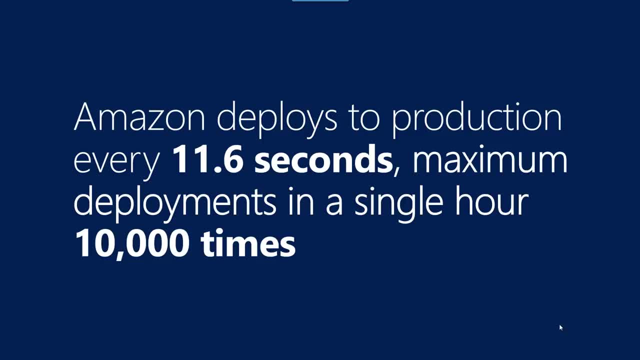 amazon. it deploys to production every 11.6 seconds, maximum deployment in a single hour around 10 000 times. and there is a great session by amazon team explaining their journey for the continuous delivery. also here there is some other example. amazon is not the only company. so we can. 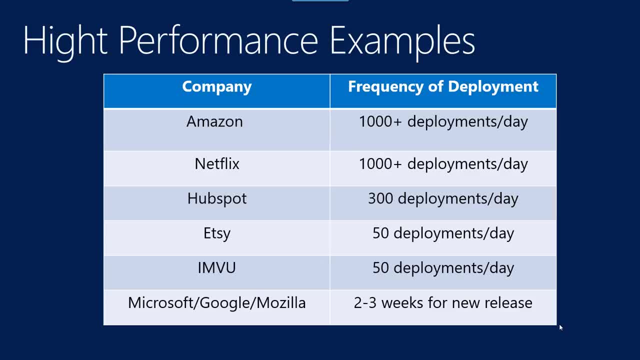 see here by frequency of deployment. we have amazon: 4 000. more than 1 000 deployment per day. netflix, zeldo, mix- that is really easy to. tutorial6 has more than 7000 deployment per day. same hubspot: 300. etsy: 50 deployment per day. imvu: 50 microsoft, google, mozilla- two to three weeks. 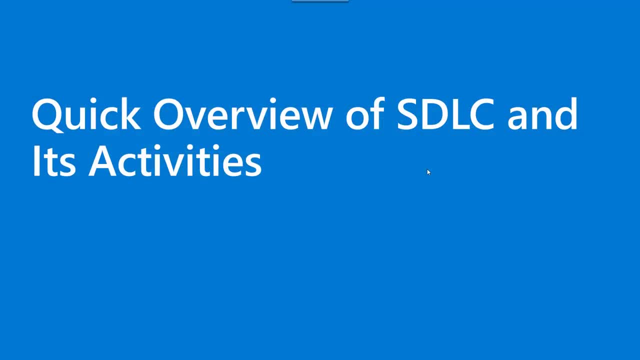 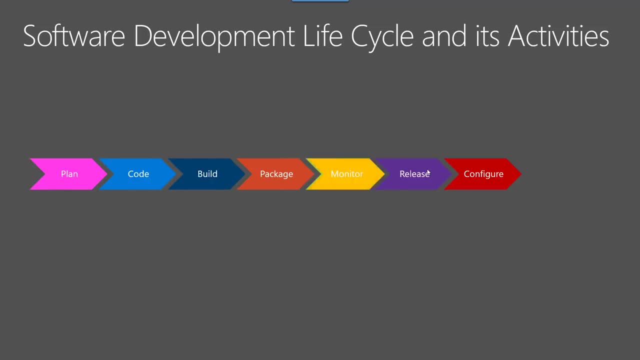 for new release. let's quickly review the software development life cycle and its activities. so as we have the sdlc, while it looks sequential, but in the modern software engineering development they are not sequential. for example, code build and test. they usually happen at the same time when we're talking about agile and scrum. but to just explain the idea, this is the the main stages. 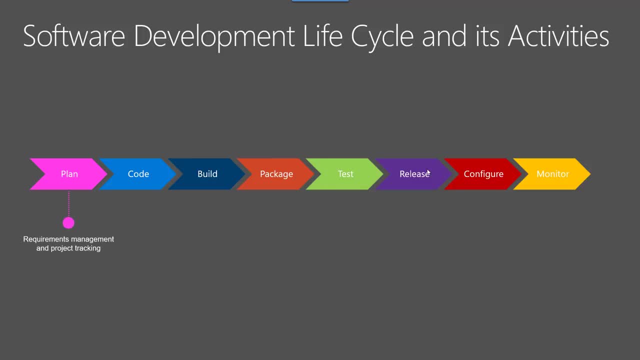 and in each state we have different practices and activities. for example, in the planning we have the requirement management, prioritize, the backlog and the project planning and so on. in the code, we have the code development, we have the version control, the branch and merge and all these practices. in the build, we have continuous 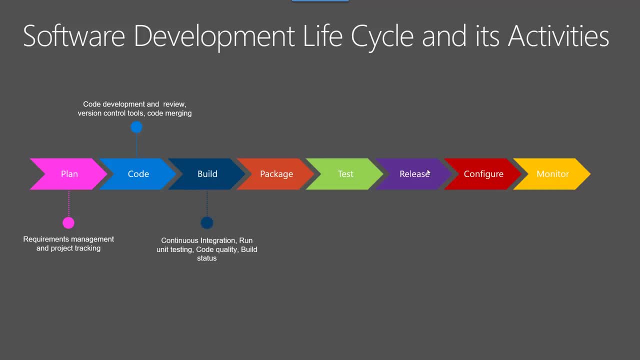 integration. we we run the code tests. the code quality is the build status in the package. we create the package from the artifacts, which is the output of the build, and then preparing the package and storing the package on the package repository. in the test, we verify the application by running. 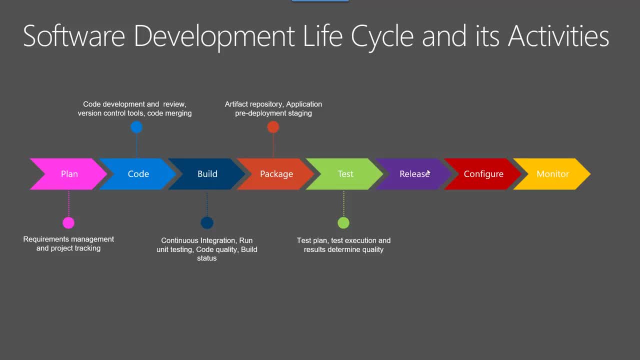 test plan, test execution and determined the test results. in the release management we we managed to deploy the application. we pick the package from the package repository and start deploying the application to the destination in the configuration management. this where we manage infrastructure as a code, configuration as a code and it is part of the source control as well. so all our 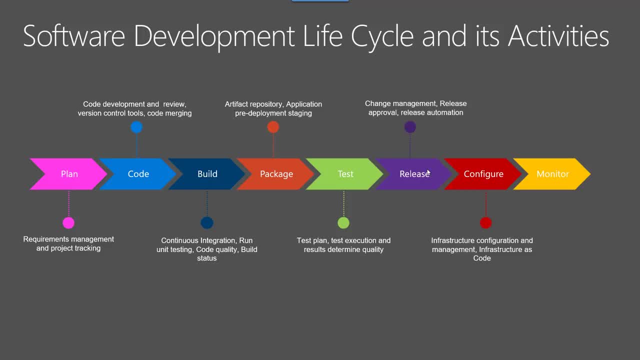 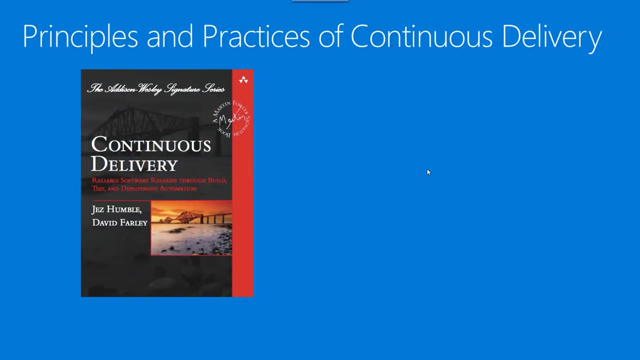 code, either infrastructure or configuration, is under source control and in the monitor we monitor the application performance and usage and experience to understand how our user or end-user using our application continuous delivery principle and practices. this is one of the best book about continuous delivery and it has great eight principles and four. 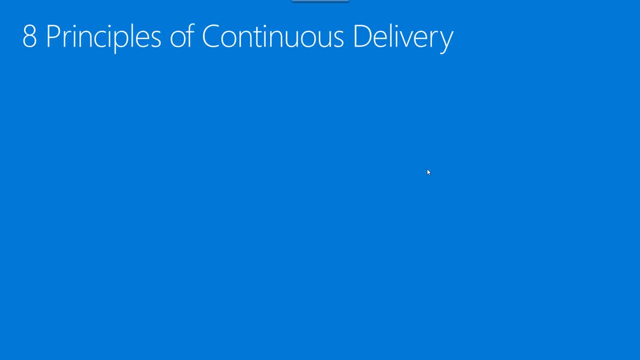 practices about continuous delivery. so let's look at the eight principles. the first one is a process for releasing and deploying software must be repeatable and reliable. it's very important to be able to to run this process again and again, but to meet everything, everything can be automated. I just have concern about the keyword. 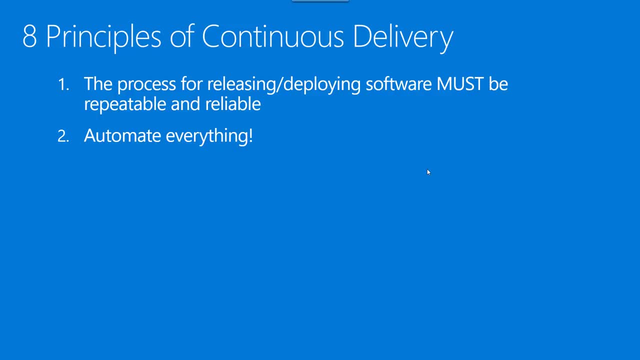 everything, because sometimes people they want to automate anything like, for example, they don't have a manual task, and then they start thinking how we can automate something which is not exist in the beginning and this is not correct. I mean the main idea for automating everything, this answer or this reply for people when they say this: 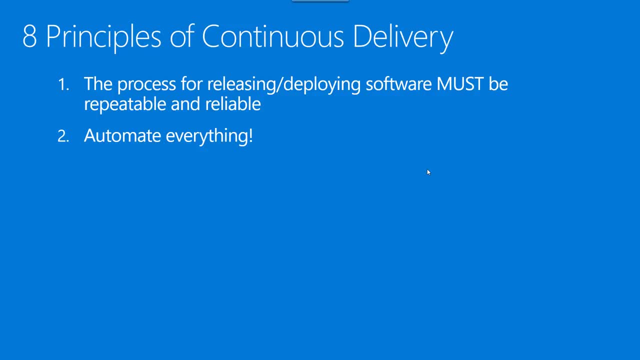 can't be automated. no, everything can be automated and we are going to automate everything. but first we want to make sure that it is repetitive. so you go first for the manual and then if it this repeated, then we start thinking of the automation, and if it's repeated again, then the automation is: is, um is a solution. 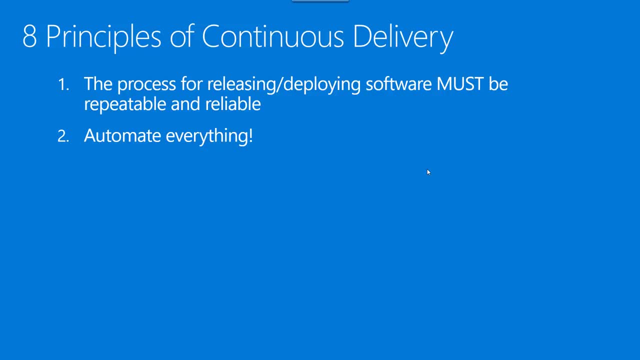 but don't think of automation at the beginning, without having a repetitive task. if something difficult or painful, do it more often again. I could spend the whole day talking about this and this is the main reason for most of the companies that they implement high performance DevOps, that they they talk less time to. 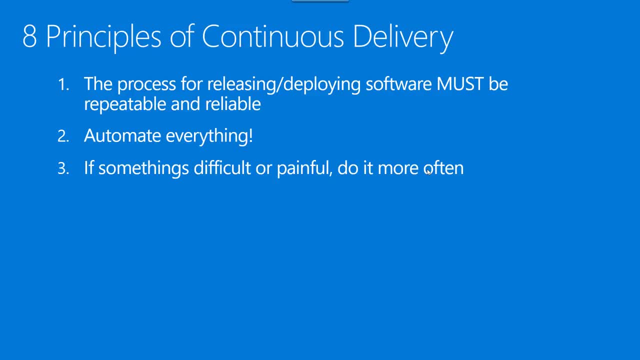 recover from failure, because they usually using this principle: because if this is painful, if this is failure, don't afraid of it. just to welcome the failure and praise the failure and just learn from it. take it as a train and you will find the way to make it very easy to you. 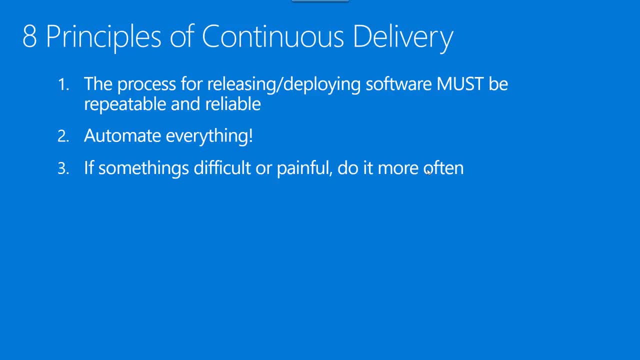 and make it, you know, something is not painful anymore. keep everything in source control. this is very important. source control. it is not for our application source code only, it's for everything. but again, I have a concern about everything, as I explained before. so in in many cases we found 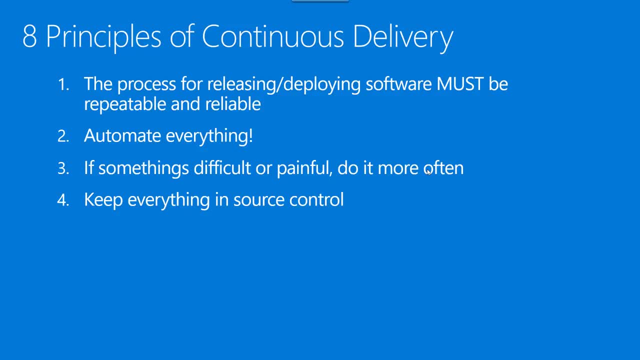 people do put under source control some files which is not belong to the source of control. so, for example, you don't put the binary under source control, you do not put the minifying file under source control. so any file that process by the tool and produced by by, by automation, it is not under source control. we only keep. 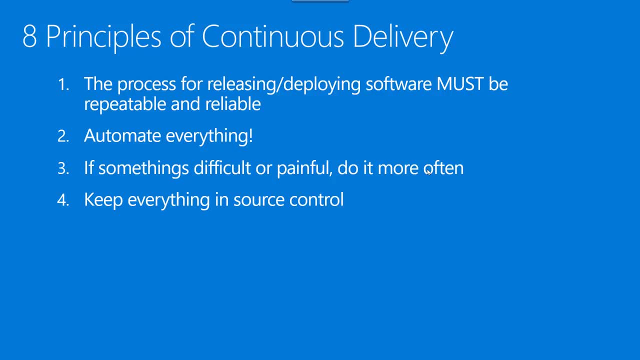 the file under source control where we edit them. but again, in some cases some of the files we don't edit because we don't, for example, we don't use infrastructure as a code, so we don't have our infrastructure as a code, so we will keep them. no, the main idea that everything you edited, either configuration or settings- 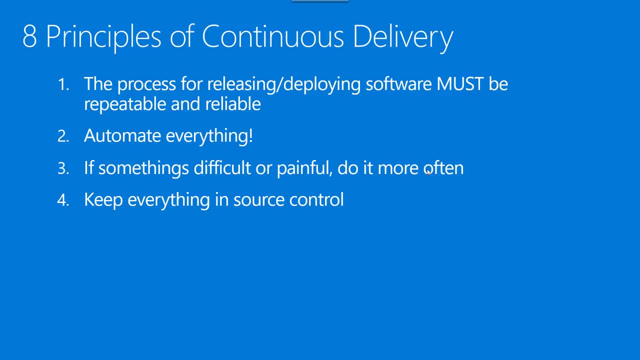 or infrastructure. it should be under source control. so, whatever you are going to change, it must be transformed into code and this code under source control. but anything that is generated, or it's an output of build process or compiling, or you don't keep it under source control for. 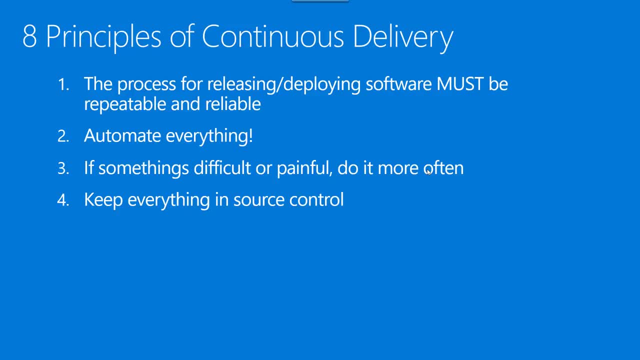 example, any generated files, it is not under source control. done means released. when we're talking about done, it means released. so when we're talking about continuous deployment, continuous delivery, it means delivery in production. build the quality in again. quality not at the end, but we're starting. 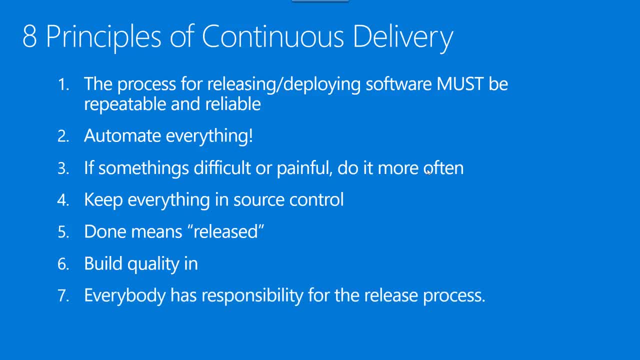 from the beginning. everybody has a responsibility for the release process. it is not the responsibility of the operation team, it is the responsibility of every one of the team. the last one: improve continuously. we we need to look at continuously improving that using the kaizen. okay, look at the four practices of the. 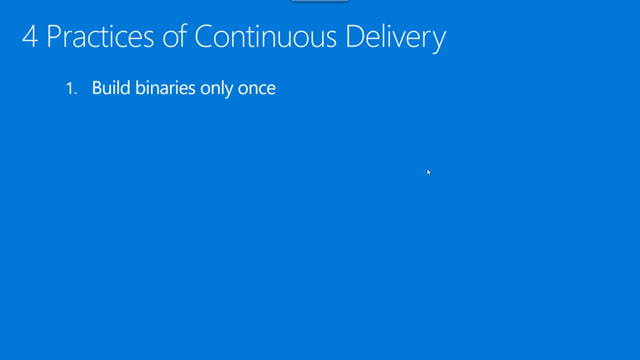 continuous delivery, build binary ones. this is very important so it is not like every time you want to deploy to as an environment, then you trigger the build and create the binary. this is why we have the package repository, where we build once and store our package in the package repository and then deploy this to different. 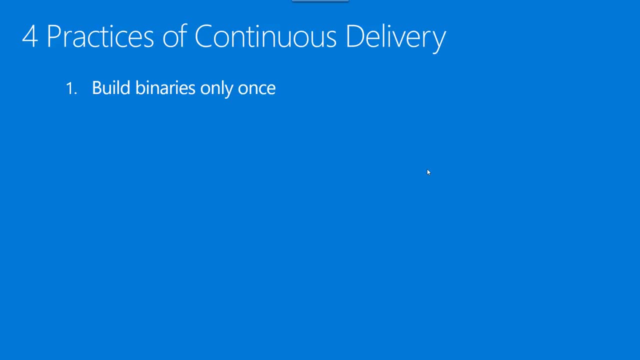 environment. so we build once and deploy multiple times, use precisely the same mechanism to deploy to every environment. this is very important because in many cases some companies they they just deploy for all environment in in one way, but when they deploy to production they're using other. so we must trust our deployment mechanism and we have the same mechanism. smoke test your deployment. 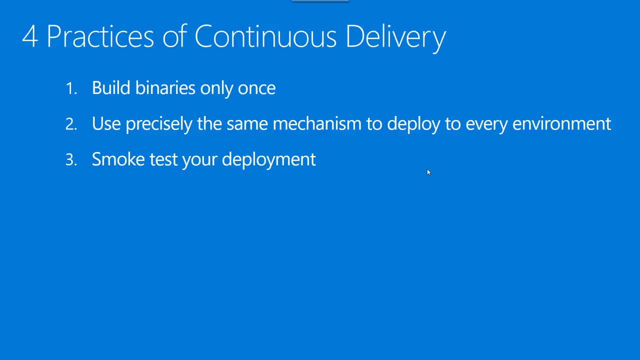 I must verify that my deployment is correct. if anything fail, stop the line again. don't cheat the process. just make sure that if it is painful, do it more often and you will learn. you will. you will train how to deal with the failure, and then the failure and the benefit will not be. 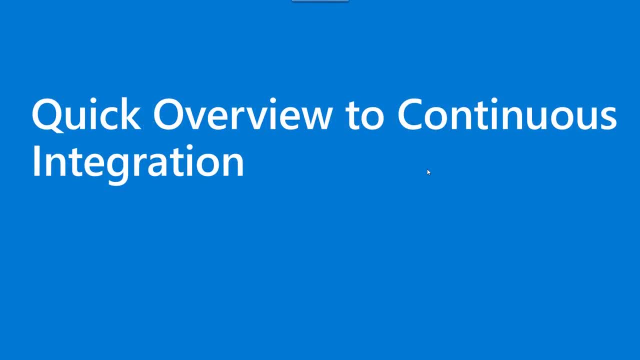 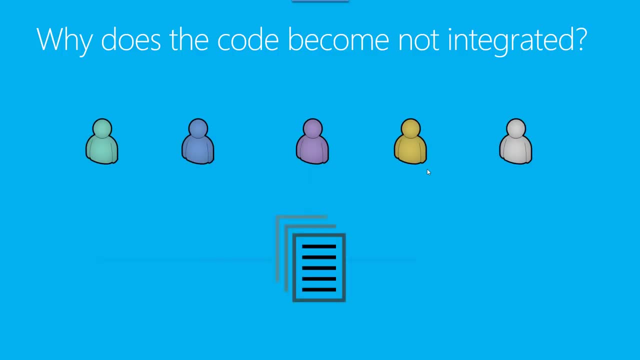 painful anymore. so let's have a quick overview to continuous integration. why does the code become not integrated? so if we have many developers working on the same code base, this is probably will have not integrated. but first let's understand what does it mean by the code is not integrated. 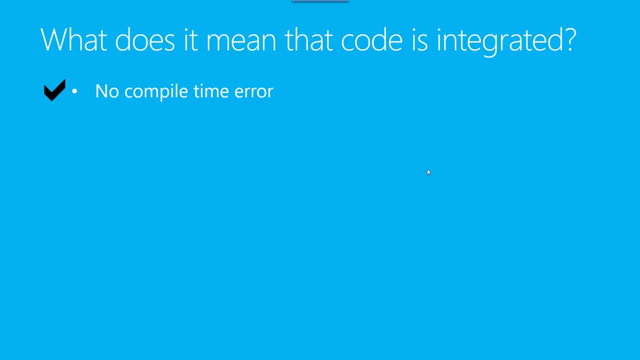 the first is, which is the minimum of the code is integrated, means that no time error. the second one, which is an optional, we usually calling that quality gates that no unit test fail. so all test cases are passed. the third one: good coverage for unit test exceeds certain percentage. so, for example, we identify that could cover. it should be uh, not less than. 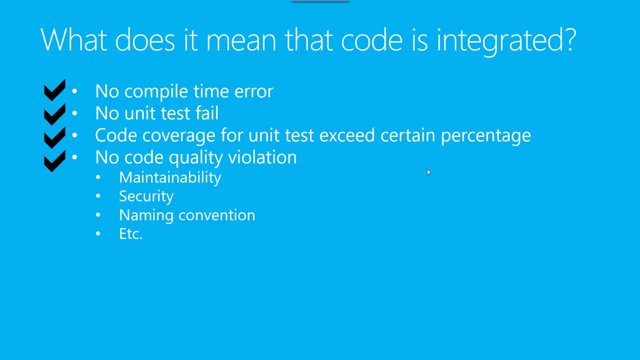 sixty percent. also, we can have that there is no violation for code quality, like maintainability, security, naming convention, uh, portability and many. all of that identifying the in the integration of the code, and it's it's very from company to other based on how you would like to keep your source code is integrated and to 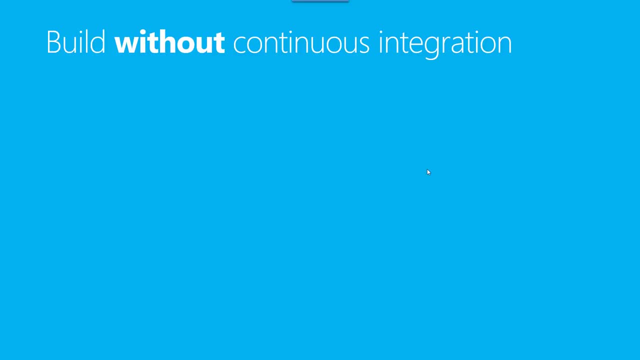 understand more about that. let's see what is the case if we have a build without continuous integration. so let's say that we have our developers and we agree that before we commit any code in the source control first we need to run all the code. first we need to run all the 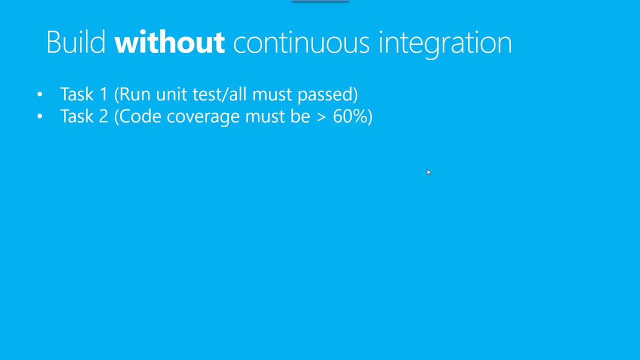 tests and all tests must pass. the second, that could coverage must be greater than sixty percent. and the third task, that code quality. all method must has lines of code less than 10 lines. so this is my specification or my requirements for for the code to be integrated. so if safe is a developer. 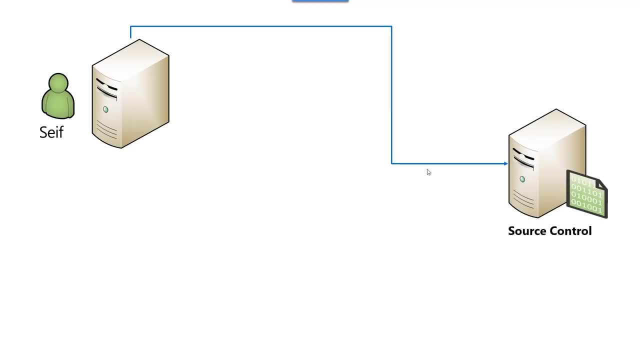 that writing the code and he commit his code and save should run the tasks. as I explained. the same for Laura when she completed the code and she want to commit and she should also run that. but for me I don't know if they run that or not. no one knows if they, if they run or not. 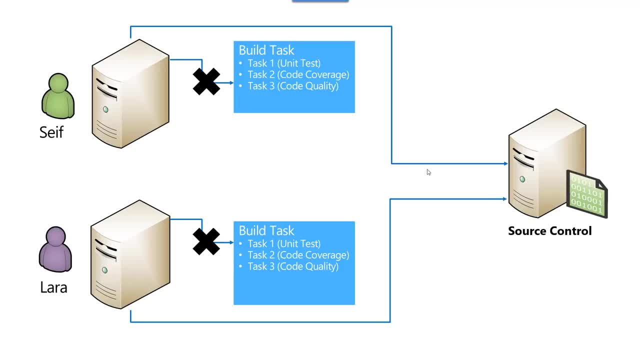 this is why they might run. maybe they forgot, maybe they have a problem, I don't know- and in this case their code will not be integrated and this will lead that one of them, or maybe both of them, will commit a code which is not integrated and we and doesn't satisfy my quality gates or 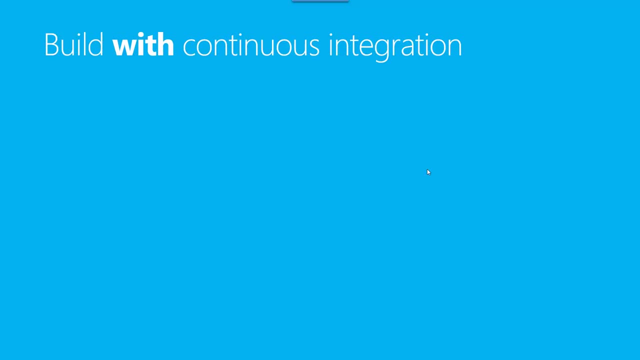 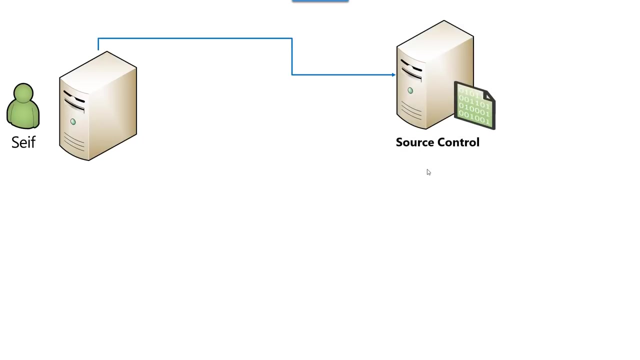 specification. so let's see the scenario with continuous integration. when I have a continuous integration, if save is a developer and he wants to commit his code once he try to do that, this will not commit the code but instead it will trigger a build server which will run. 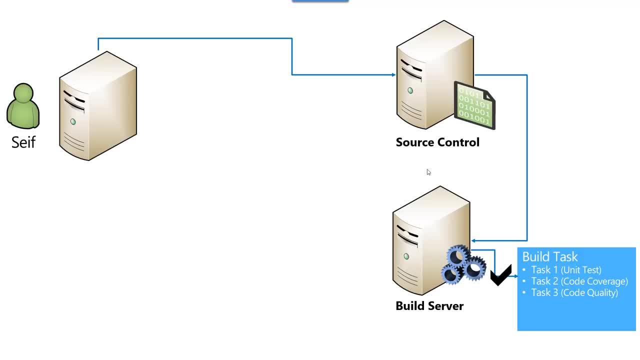 all the tasks run the unit, test the code coverage, the code quality and review them and make sure that they passed. if they passed, then the code will be committed. if they don't, then the build will fail and it will prevent the code from committing to the source code. the same will happen with 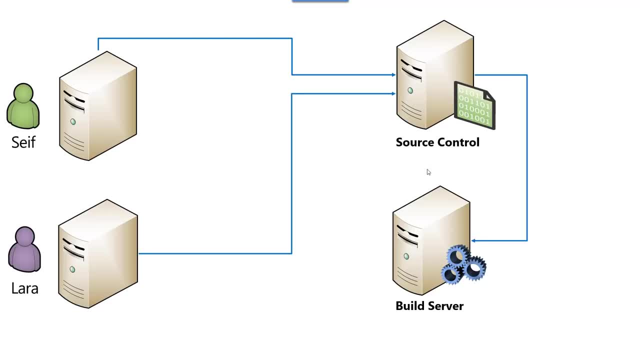 Laura, if she want to commit the code, trigger the build, the build run and run all the specification and the verification, the checklist, and pause, this will will commit. if it's fail, it will prevent the code. this is why, if any one of them or both of them run, 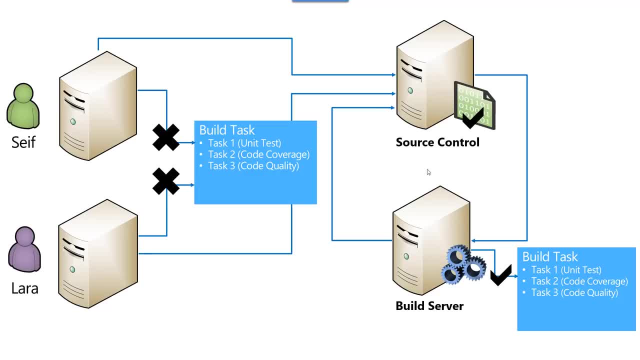 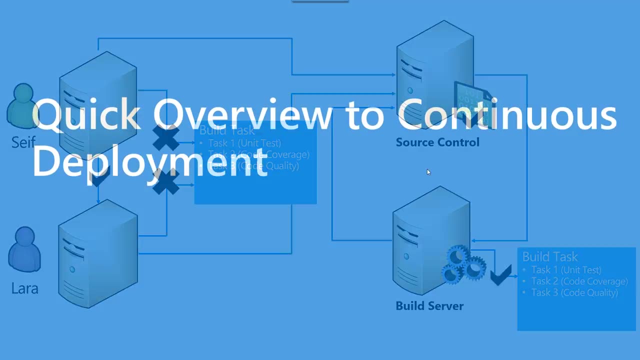 or not, I don't care, because at the end, my source code is guarded by the build server, the build server working as a safeguard for the repository or for the source code, and my source code always integrated according to my specification about the code. so let's have a quick overview about continuous. 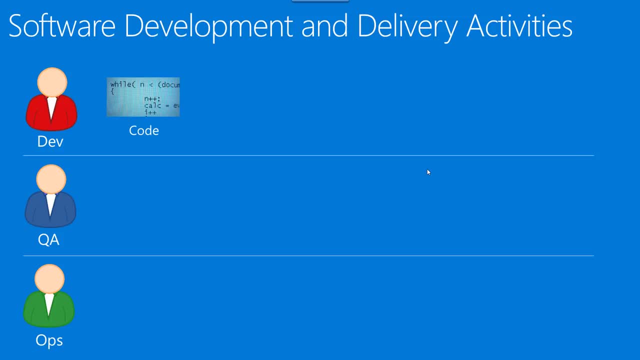 deployment. we always start writing code, which usually a high level language like C sharp, for example, and then they start kick the build or start building the application, and the build will produce the artifacts, which usually is the transformation of the source code into, if this is a desktop. 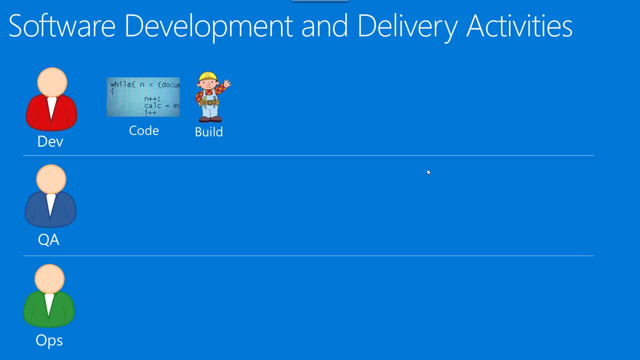 application, it will be machine language assembly for, for dot net, for example, or if this is web application, this could be minifying JavaScript and CSS. sometimes you should add code in the web, because I think Robting is a great way to do that and he is connected to influence by cloud zero. 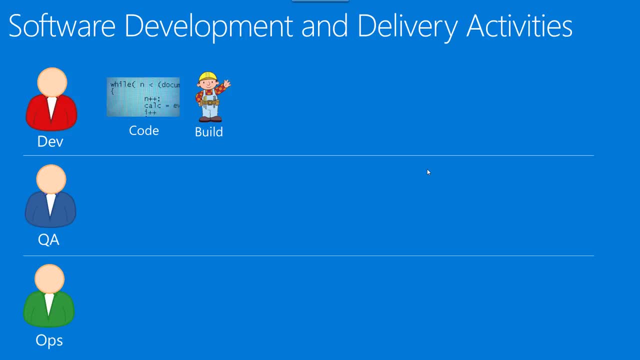 Sometimes it could be bundling JavaScript. The main idea of the first step of the build is to transform the high-level language into a language destination specification And, of course, the build can have many tasks, as we explained, like run the unit test, for example, and code quality and so on. 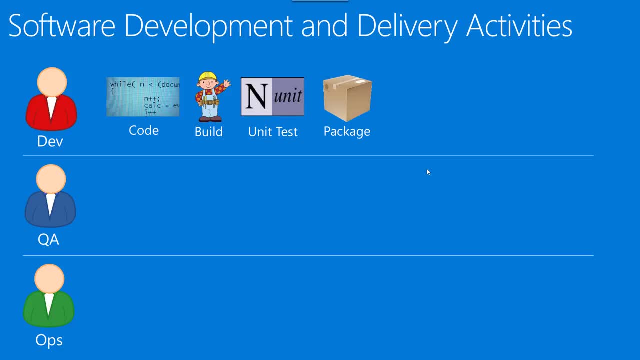 And usually the last task of the build is to once we have, as we explained, the build is creating the artifacts. As we have the artifacts, the last task is to package this artifact, And the main idea of the package artifacts is to organize these artifacts. 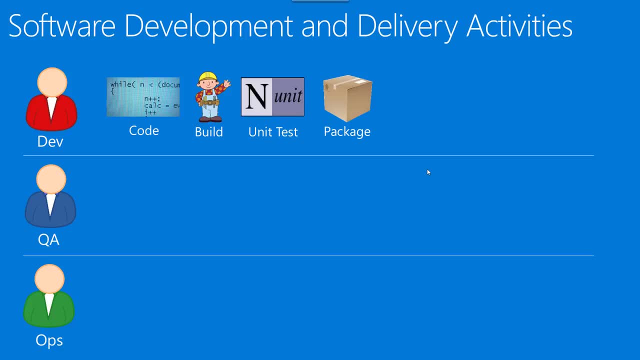 into a package. Just, it's a matter of organizing these artifacts in a way, boxing them to be easy for distributing or redistributing. Once I have the package, then I start provisioning the destination, Creating the environment and preparing the environment, And after that I pick the package. 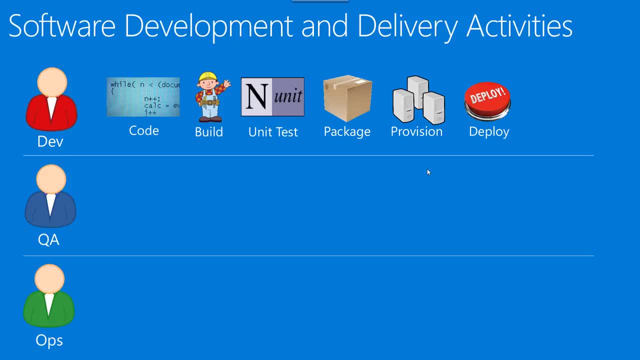 and then deploying the package. This was in the old But now the best practices recommended that before I doing the provision and the deployment, I should store the package in the storage, And this is exactly what we are going to use: the package repository. 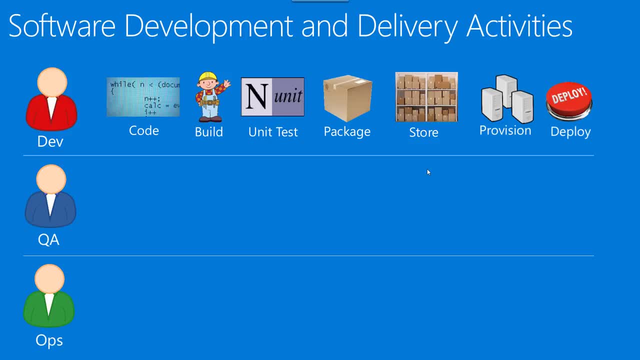 So, once I store the package and if we remember the four practices of the continuous delivery, build once and deploy multiple times. This is exactly what we will do when we store our package, Because we are going to store the package in the store. now we deploy to the dev environment. If I want to deploy, 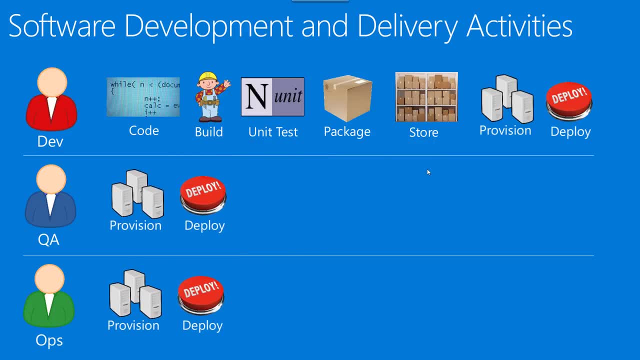 the QA or the pre-production, then I will just pick the same binary, which is the same package, from the storage and start deploying that, of course, provisioning the environment first and then deploying that. So, build once, deploy multiple times To move from one environment to another. 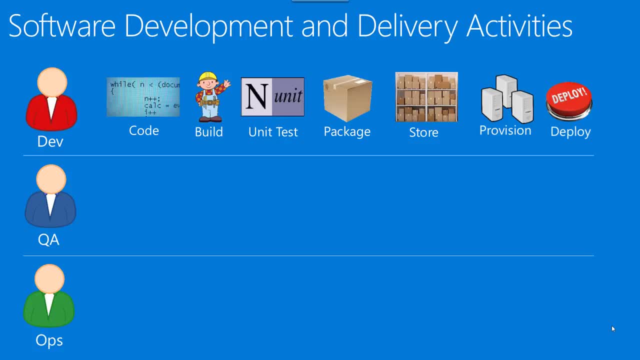 usually it requires approval And we have two types of approval: the pre- and post-deployment approval. So the pre-deployment approval, it's like sign in to receive, and the post-deployment it is like sign off for completion. 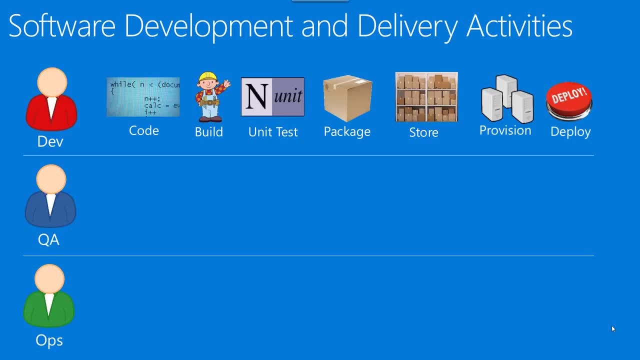 So, for example, if we are in the dev environment and after deploying to the dev environment and everything is fine, then it's required some of the developer- or maybe the dev manager, according to the process that to sign off that the development complete. Once this is completed, then 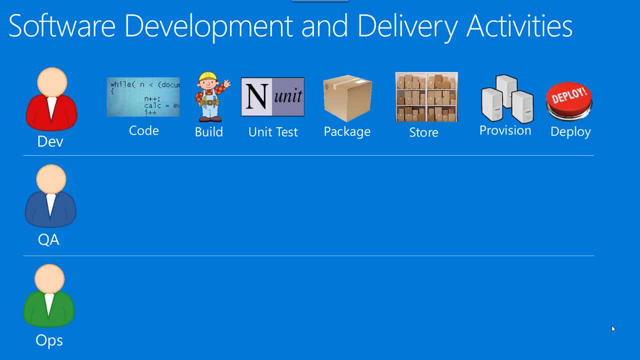 the QA needs to have a pre-deployment approval So they sign in that they receive the build to start working on the test. Once the QA approve in, then the deployment to start and of course this will start by provisioning picks, a package from the storage. 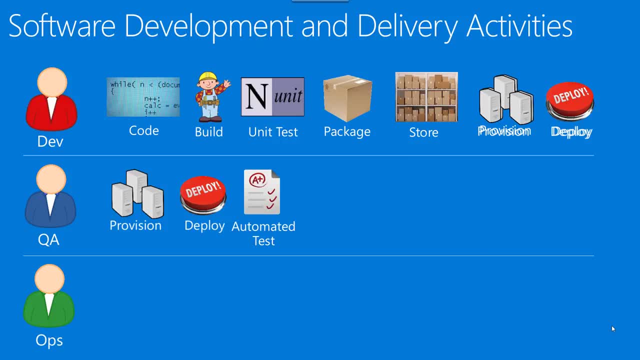 deploy the application, then after that run automated acceptance test and maybe run some manual test at the end, And once it's completed, then the next step is a post-deployment approval, which means that the QA completed the work and they sign off and the same. 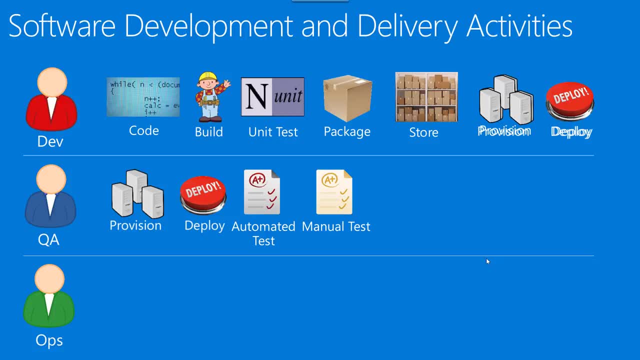 for the next stage, there is a pre-deployment approval. Once it's approved, then the environment will provision and deploy. If this is a pre-production, then there is a post-deployment, which means that we sign off and ready for production, and so on until it reaches the production. 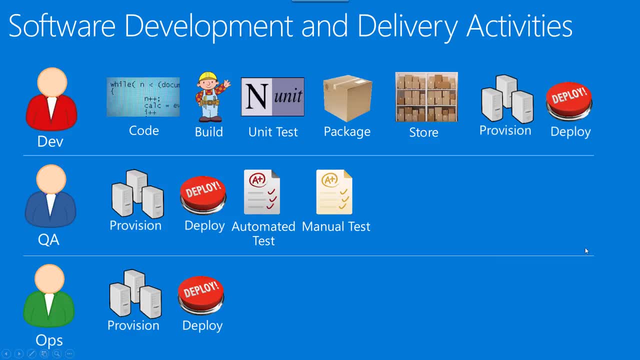 which means that there is no post deployment as the application will stay and will not go out as there is no next stage. So let's look in details for the risk management steps for one stage, starting from the pre-approval deployment and the post-approval deployment. We will take the QA as 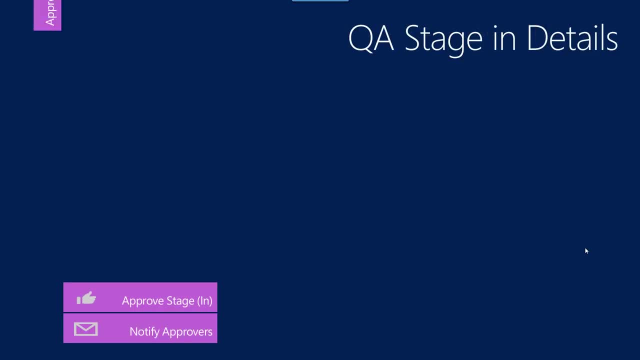 an example. The stages start by that, the QA receiving the notification for approving that the development completed and they are ready to approve, so the deployment can start. Once the QA approve, then the deployment starts and the first step is to provisioning the environment- This part 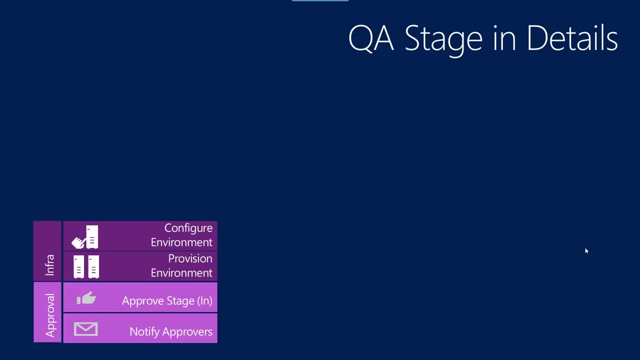 of the infrastructure is the code. so usually the deployment or release management picks the source code for the infrastructure from the source control and start creating the environment or provisioning the environment based on the infrastructure instructions which exist in the code. Once the environment is completed, then the next step is pick the configuration as code and start configuring the environment. 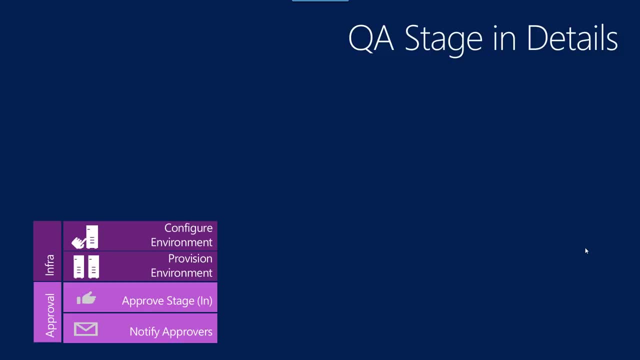 And this is the post-configuration. For example, if provisioning the environment is a virtual machine which has Windows server and then configuring the environment is enable IIS Windows feature or maybe enable ASPNET or maybe open port on the machine. So a post-configuration is needed for the environment, but we need to provision the environment first. 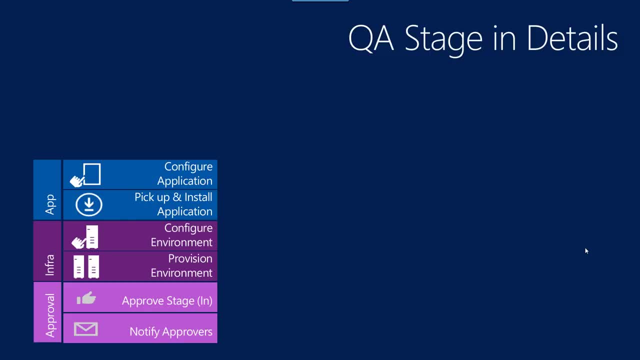 Once this happens, the release management starts to pick up the application from the repository, from the storage, then starts to distribute or install that on the environment. Once it's completed, then the post-configuration for the application. Maybe we need to create some data lookups, data all this kind that is needed for the application. 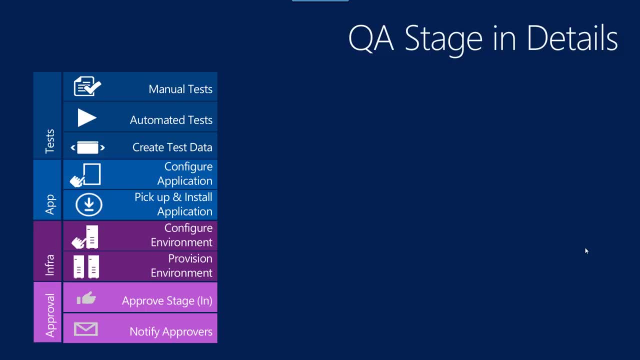 Once this is completed, then the release management will start creating the testing data, Because to run an automated UI test you will need data. For example, if you want to test that the registration is successful, then you need to have a username, a password email too. 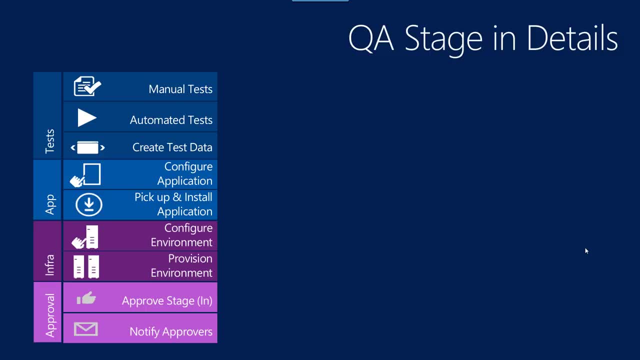 You can try that with different scenarios. So the first step in running the automated test is creating the test data, then running the automated test. Once this is passed, it means that The environment ready for manual test. then the QA go and start running the manual test. 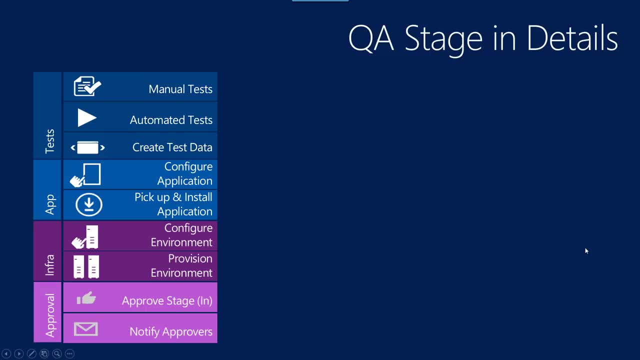 Once they approve the manual test, everything is fine. they sign the stage, which means that the application is passed all the tests, And this means the sign-off, which means that this will trigger the notification for the next stage- approval, of course, usually by email. 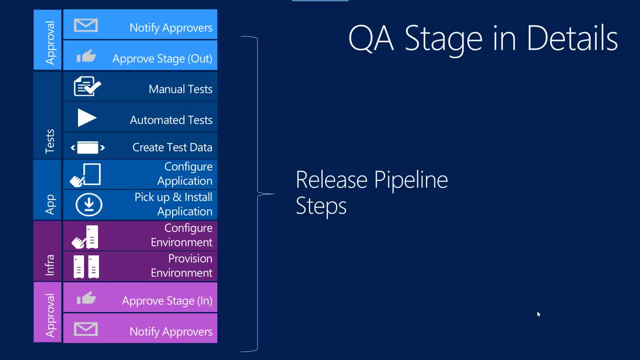 So this is the release pipeline steps And, as we saw, the release pipeline Doesn't include creating artifacts or package or store package in the repository, But release pipeline is responsible for running automated acceptance test And creating the package and all these tasks is part of the build, not the release. 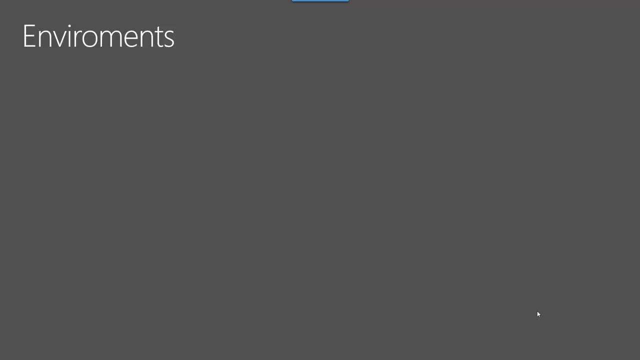 So let's look in more details about different environments and the process for moving the package between one environment to another, which we calling promoting the package. We usually have different environments And this could be different from one organization to another, So this is just an example. 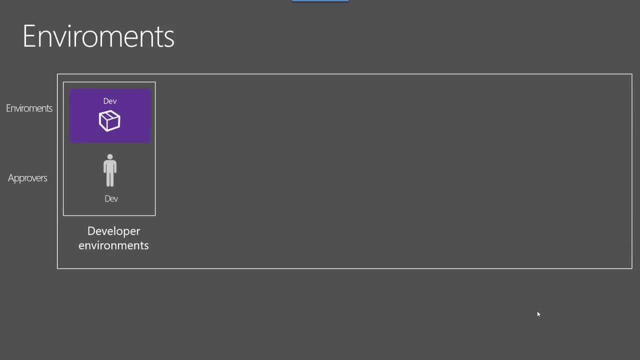 The first environment, which is the development environment. This is usually the environment where the developer start verifying that the development is complete. We have two approaches here. The first is that consider each developer machine is a developer environment, Or in some cases it may require having a development server. 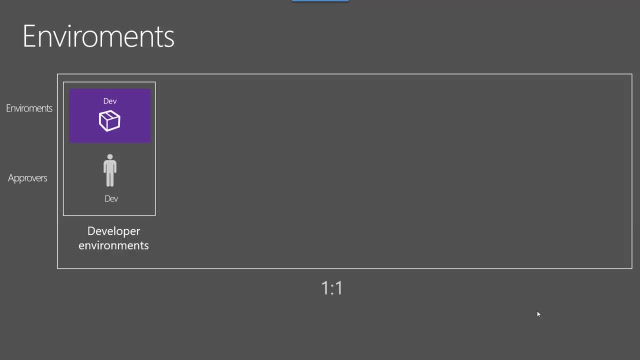 The main problem is that. The main problem is that. The main problem is that If it is required to have a development server, don't make it as a bottleneck, Because this is the last step before moving to the next stage And if you have one development server, then this will make a bottleneck. 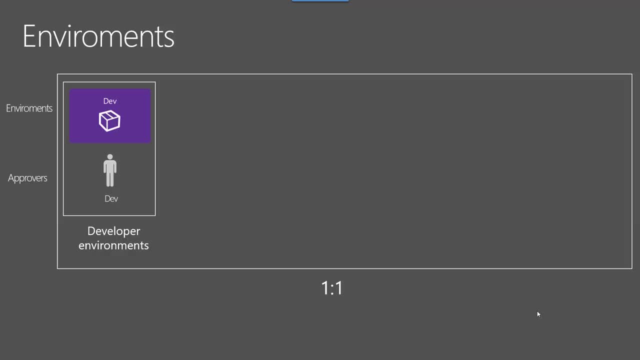 Because, for example, if another developer want to deploy to the dev server but it's not available because it's occupied by another one, This will make a problem. So we should have like one-to-one relationship between developers And development environment. 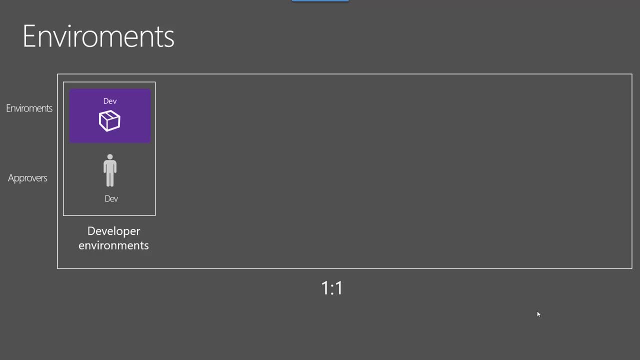 And this is not only for development environment, but for every environment. We should not have a bottleneck, that the environment is not available. You may be asking now how we can have many environment. If you remember, we agreed that we provision the environment on the fly. 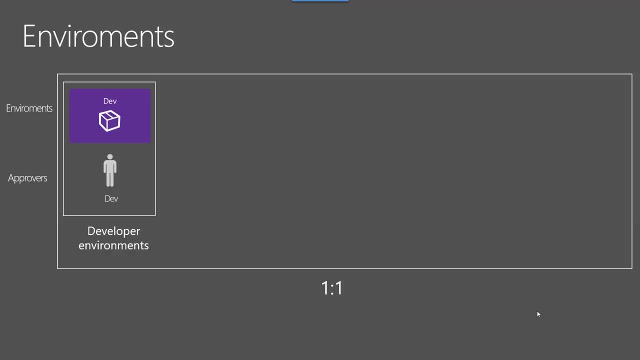 And once we complete it we can tear down. So once the development is complete, then the approver here is the developer. The developer sign off that he completed. He completed the development. once he did that, then the package is deployed to the testing environment and this will be for what we call the feature test. 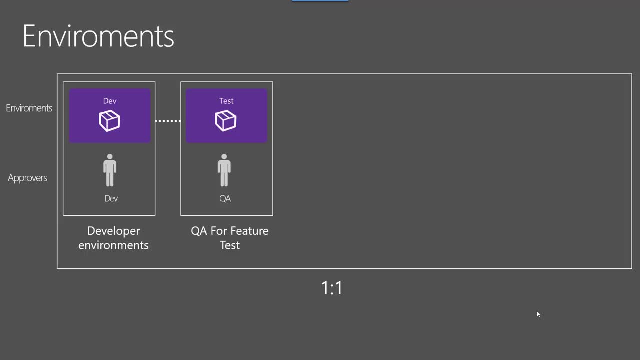 This testing environment is very important and the feature test process is very important, especially if you don't implement feature flag. Feature flag is another topic. We will talk about it in another videos, But for now, just remember it is very important to have separate and isolated environment. 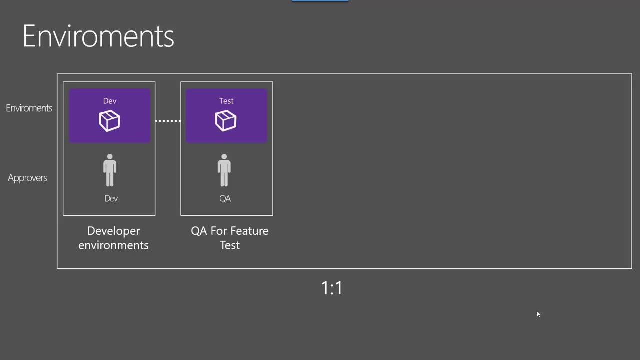 For feature test before we merging the code. Once the QA approve that the feature is completed and it's working fine, then we'll deploy the package to the QA environment. In the QA environment this will be incrementing this feature with other completed feature. 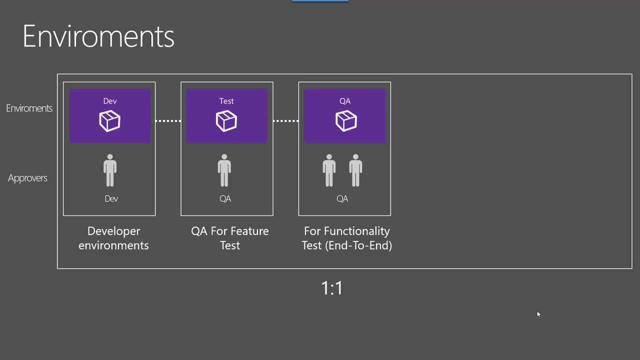 So the QA team can work as an end-to-end. So here is an integration testing between different features before promoting that to the next step stage. once this completed and the QA approved, this will lead to promoting the package to the next environment, which usually is the pre-production. in the pre-production we usually try to have some 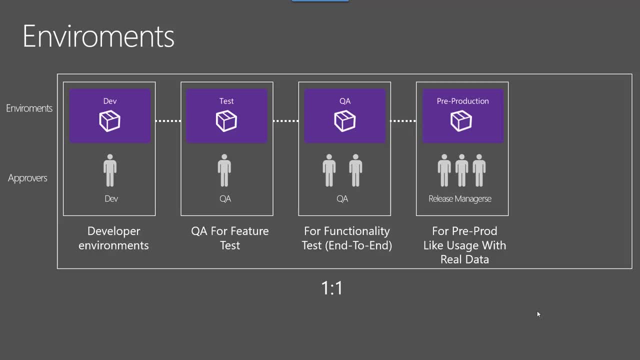 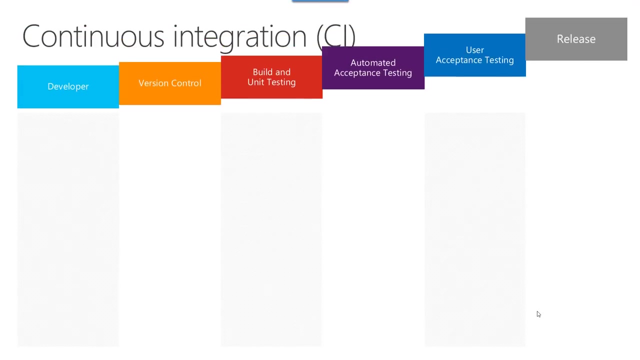 of the real data from production, of course, after we clearing is a sensitive data, so we can verify the application with with the actual data, which very important. then once the pre-production and the release managers approve this package, then the package will be deployed to the production. let's look at that from a different angle to make more sense. when the developer is starting. 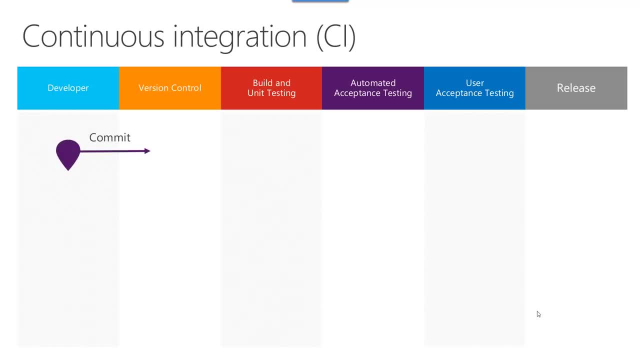 committing the code to the source control. source control will trigger the build automation and, if you remember, the build automation will start creating the artifact, the package and all this and maybe the unit testing will fail, which will bring the feedback to the developers that they need to fix. 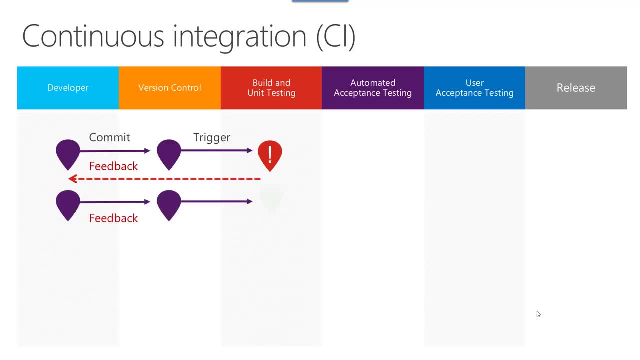 once the developer fixes that and start committing the code again- and in this time the unit testing passed, all my quality gates passed- which will trigger creating the artifacts, packaging the artifact and the store, the package in the repository. once this happened, this will trigger the deployment by triggering the deployment pipeline, the deployment to start by pick up the 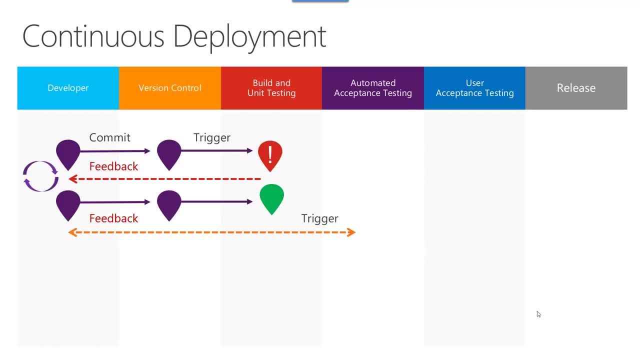 package from the repository and the start provision. the environment deploys the package to the environment and the start run automated acceptance test. if the test fail, then this will get a feedback for the developers. so the developer now needs to fix the problem. then, after the developer fix the 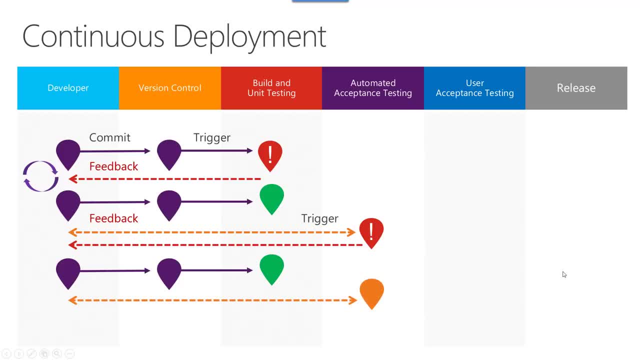 go through the steps from the beginning. once the automated test has been accepted or has been passed, then it will wait for the approval from the qa to approve and sign off to promote the package to the next stage. once they approve again, it could be approved automatically once they. 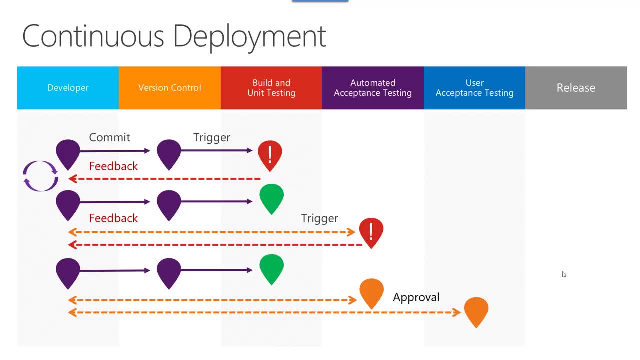 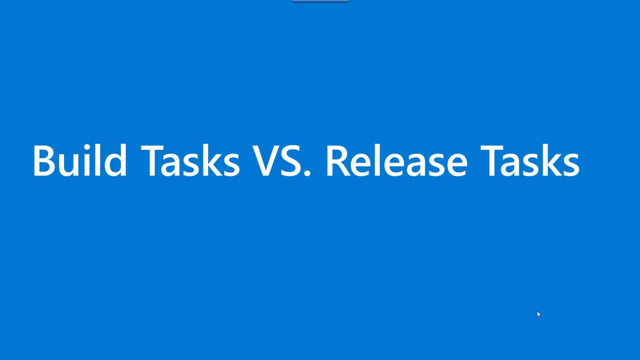 approve. it will promote the package to the user acceptance testing environment and it will wait again for the approval to be deployed to production. once this happens, here is the gate for the approval. this will deploy the package to the production. so now let's review and make sure that we we can distinguish between the build and release task, or the, the build pipeline and the. 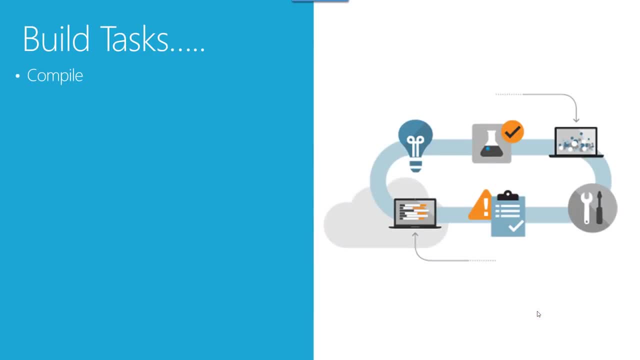 release pipeline. so in the build we we usually compile the application or bundle and the minification, any form of transforming the source code into machine specific or a destination specific language, for example. bundle and minification. the bundle here for usually for the javascript. so in the development time i will need the all the javascript in a readable form. if i have 100 javascript where 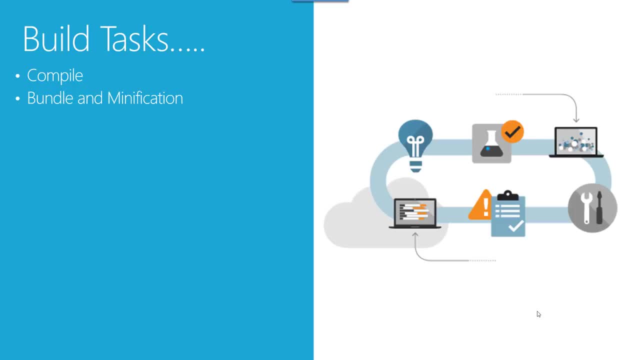 i can edit them as a developer. i don't need to distribute them to the server as a 20 file in the bundle. it will just making one file that contain all the javascript code, for example, because it doesn't need it for the server that hosts the application. for example, the same for